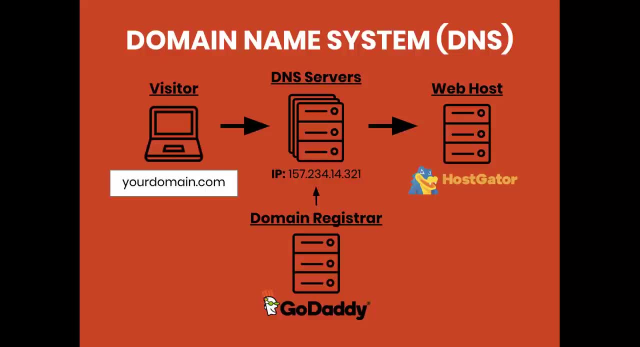 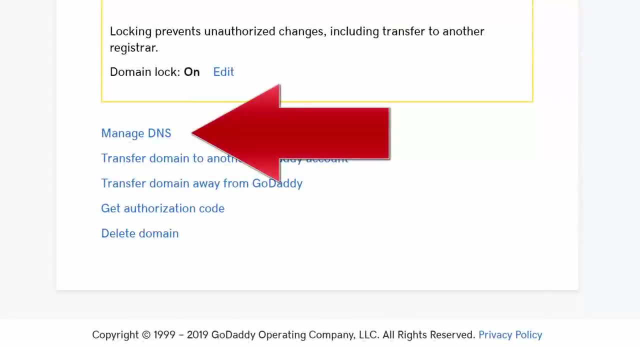 but I've had no problems with them, just for domain registration. So when you register your domain with GoDaddy, you're going to get access to these DNS settings for each domain that you register. And then when you sign up with a hosting company like HostGator, they're going to send you their DNS servers. So you sign up with your HostGator account and they're going to send you- likely two DNS servers. All you have to do is go into your GoDaddy settings and plug in your HostGator DNS servers. That's literally all you need to get set. 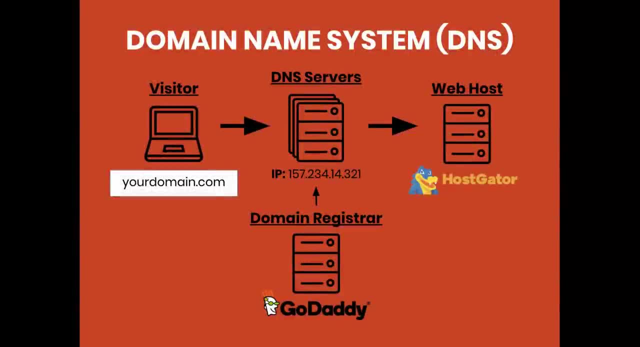 up with your website And the DNS server. its function is to translate your domain into an IP address. So all it does is when you, as the visitor, go to a website, you open up your browser and type in a domain name, it's going to send that domain name to a DNS server where it maps it to the IP address of. 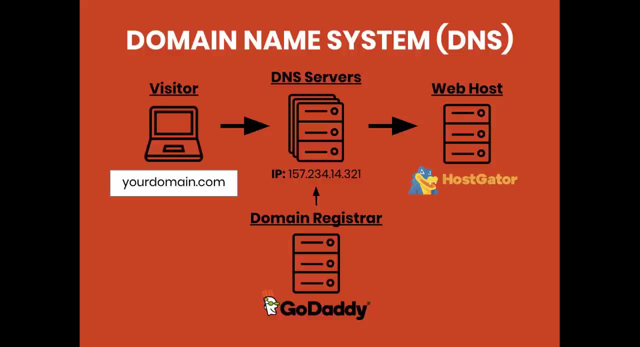 your web host and that's where it gets all the files from. So that's how the website is downloaded. So hopefully that wasn't too confusing for you and I hope that this graphic is simple enough to understand. But really, all you need to remember is that when you register your domain, wherever you register- 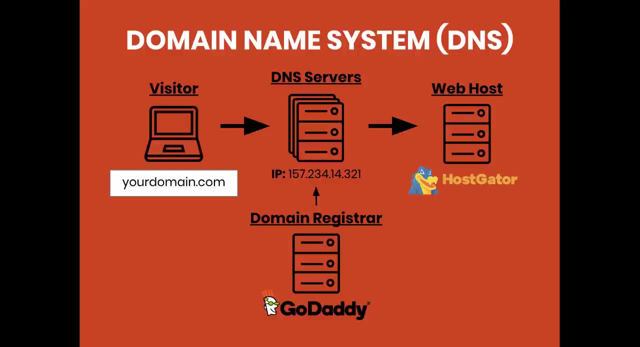 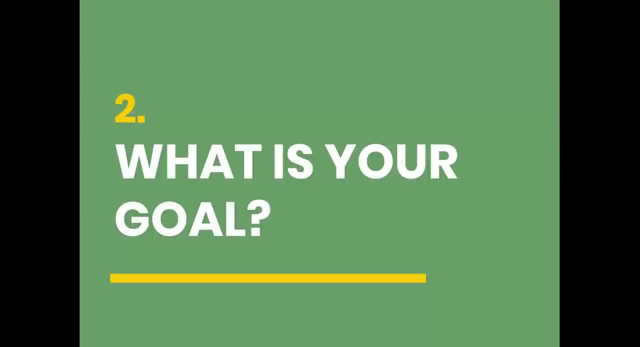 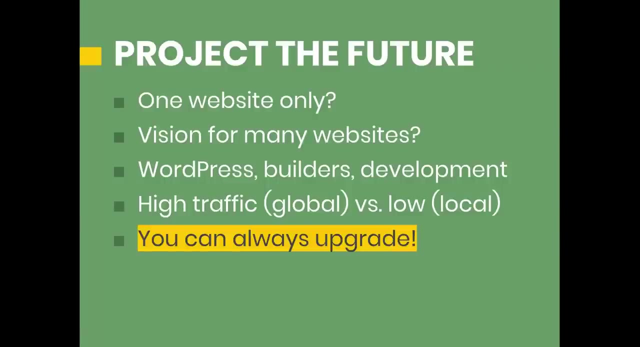 the domain, you should have access to DNS settings, and whatever you put within those DNS settings that's going to define where your website is hosted. Now, before we go into the hosting packages, we have to figure out what your goal is. You might be wanting to do one of many things, So 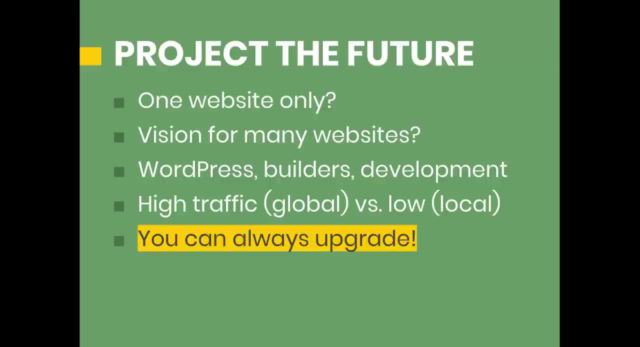 the first questions that you're going to want to ask yourself are: do you want to create one website only? Do you want to create one website only? Or, if we project into the future, are you planning to build multiple websites And does multiple? 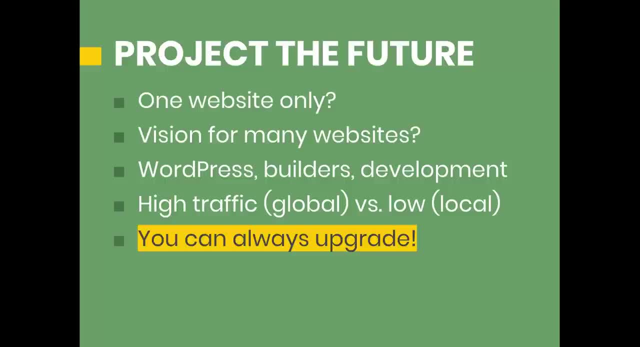 websites mean two or three, Or does it mean maybe 10 or 20?? And then you have to think about the software that you're going to use to build the website. Are you building from scratch with HTML? Do you want to use a content management system like WordPress? Are you just going to use templates? 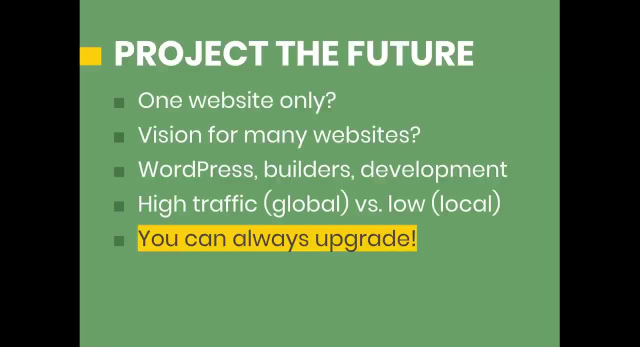 or a builder offered by the web hosting company like HostGator or GoDaddy, Or are you planning on doing custom development and maybe even code with a higher level language? So if you're just starting out a website, it's not going to have high traffic. It's going to take. 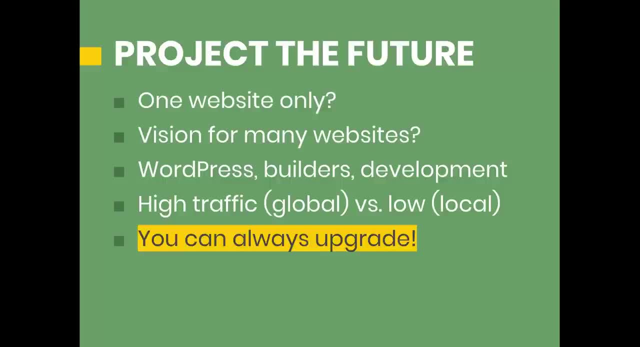 a while to build up the traffic, And then even for established websites, they might be low traffic if they're local, And then on the other end of the spectrum you might have a global oriented website based around a hobby or a general interest that applies to people worldwide. 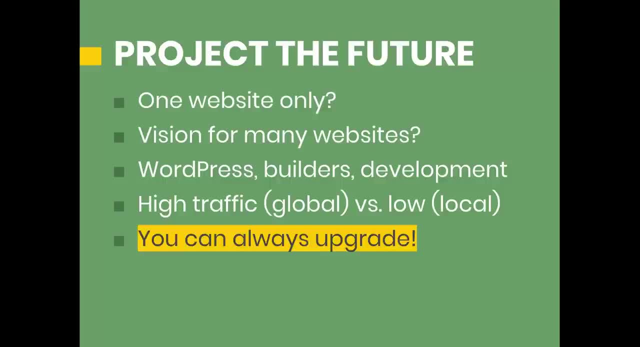 And in those cases, once you get to a point of high traffic, your web hosting options are going to be low. traffic going to change And I have to point this out. You'll see a lot of people that leave bad reviews for cheaper web hosting companies. They're people that don't consider the beginner's experience. 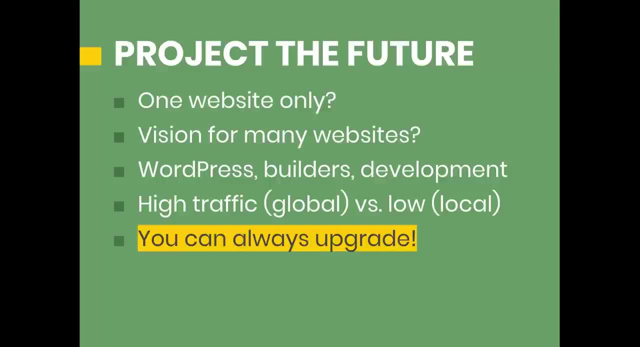 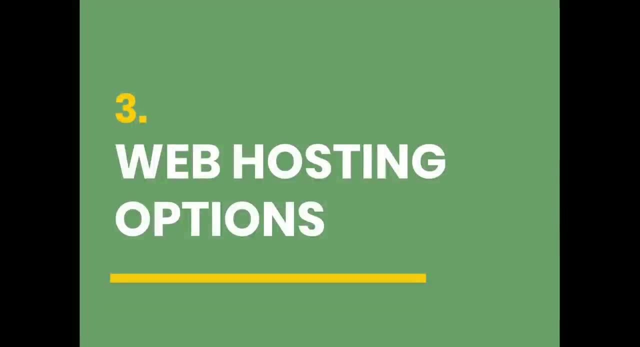 You know you can always upgrade. There's nothing wrong with starting with a cheaper package and upgrading down the road when you start getting more traffic. So let's look at the options that are going to be available to you on the majority of web hosting companies across the internet. 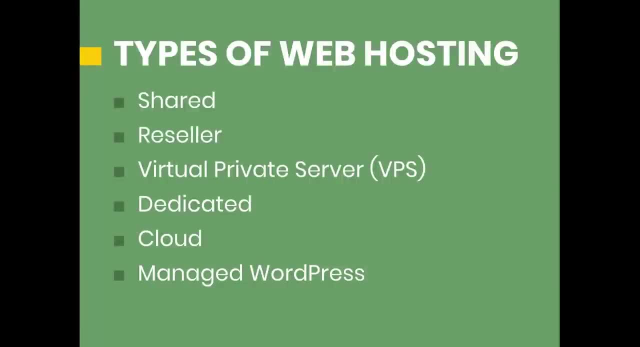 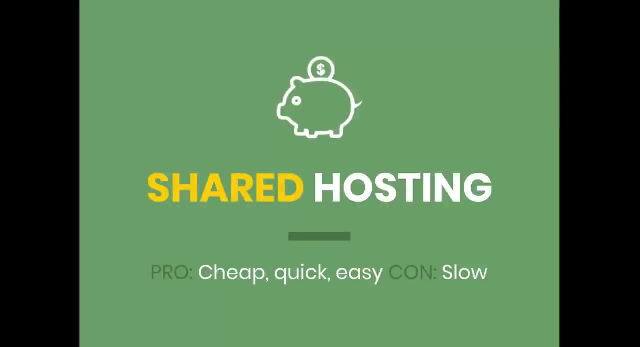 More than likely, you're going to be choosing from one of these types of packages: Shared hosting, reseller hosting, a virtual private server, dedicated hosting, cloud hosting and managed WordPress hosting. The first one is shared hosting, And this is the cheapest. 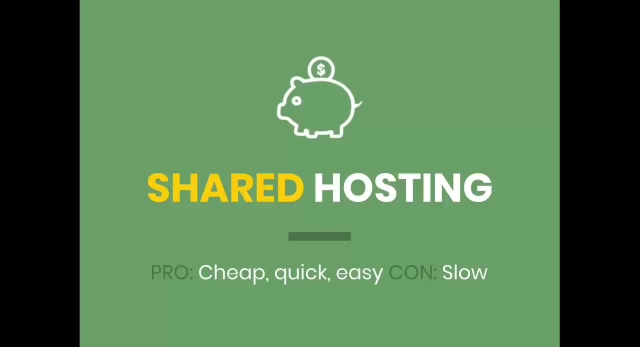 the quickest and the easiest to get started. You're going to see really great deals for shared hosting packages, And this is really dominated by the big companies. I mean, it's not just the big companies, It's the big companies. It's the big companies. 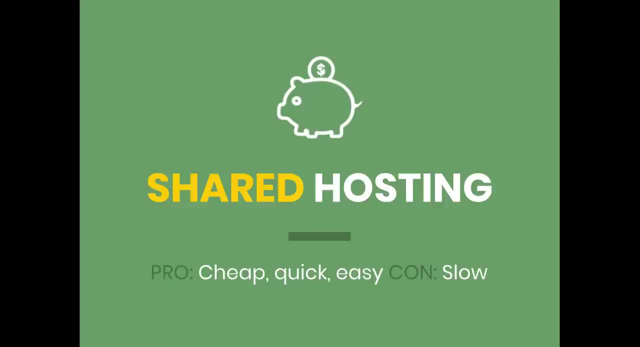 I mean, that's really how all markets are. Anything cheap is going to be dominated by big companies, And anything that's really expensive is by small companies that offer a high-end customer service experience. With that said, the main con to shared hosting. 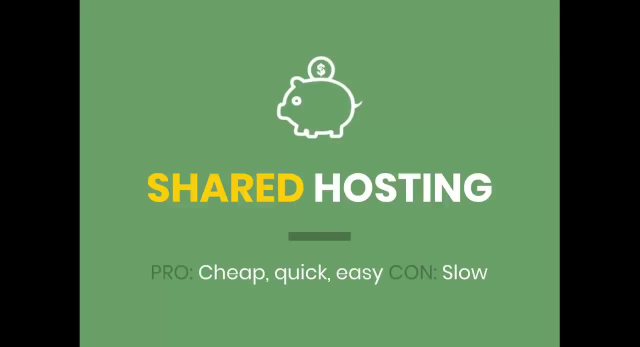 is that, as the name suggests, you're going to be sharing your hosting package with a lot of other websites. Depending on who your neighbors are, that might mean that your website is going to load slower Now. with that said, I think it's the option that you should start with if you're a 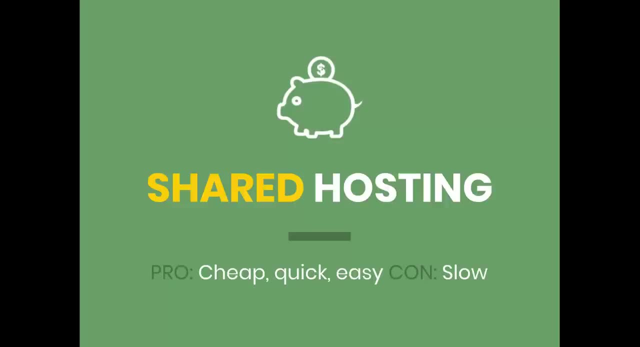 beginner for the reason of it being cheap and that you can always upgrade. The next one is reseller hosting, And this is what I started with many years ago. I had the vision that I wanted to create websites for small businesses and local businesses, So from the get-go I knew that I. 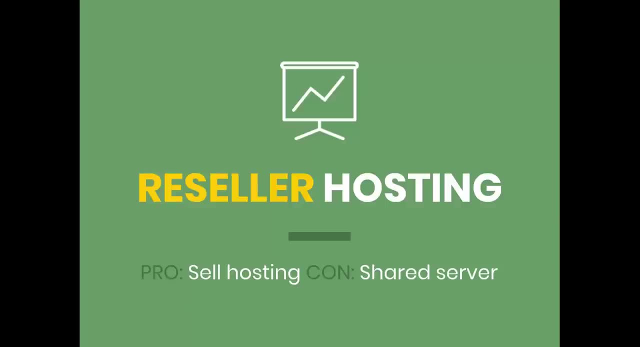 wanted a plan where I can create multiple hosting accounts, And that's really what reseller hosting is. It's pretty much shared hosting, but where you can create unlimited websites And, as the name suggests, you can actually sell hosting plans. You don't need to create websites. 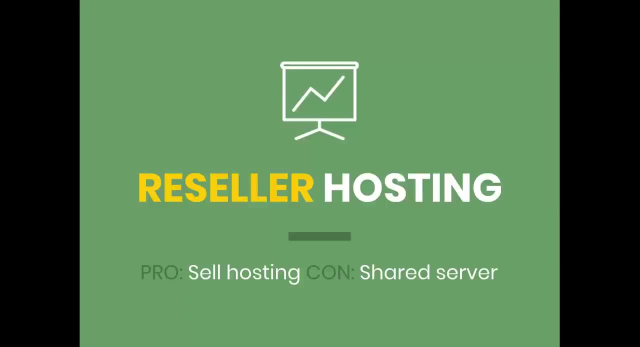 specifically, You could literally just create hosting accounts and let the people figure it out themselves. A step above that is VPS hosting, And this is virtual private server, And with this, you're getting resources that act like your own, So it acts as though it's not being shared with. 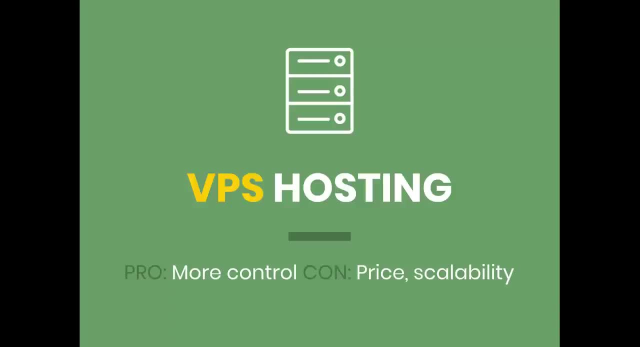 other websites, even though from a physical perspective, it might literally be on the same server, But there's software over top of it that give you dedicated resources to run your website, So you don't have to worry about other websites interfering with your performance. 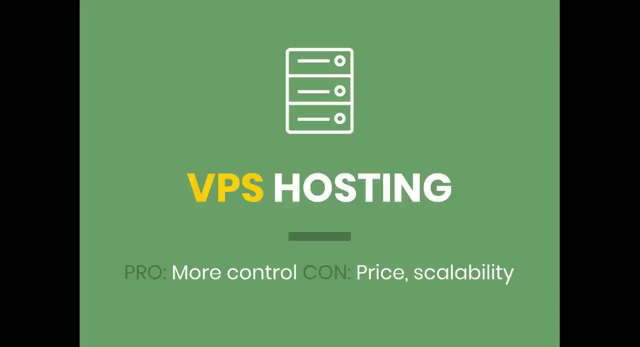 They also give you root access. So if you need to do any technical stuff or IT level stuff, you're going to have more options with a VPS server versus a shared hosting server, And the main downside is that this is going to cost more than shared hosting. 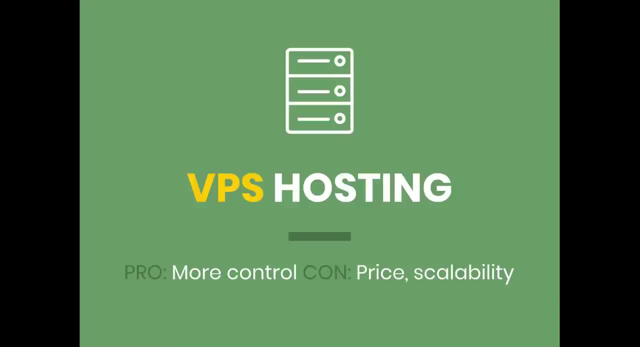 And it's also not as scalable as some of the other options. if you do start to get more traffic, So let's get started. One step above VPS is dedicated hosting, So this is where you actually get physical resources. You know, you get a physical web server that is all yours and that's where your website runs. So 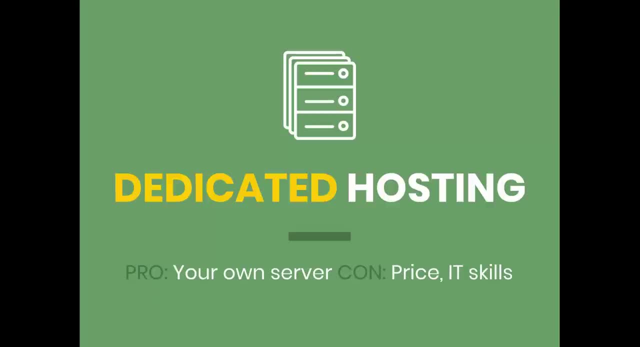 this is generally expensive. I think. I've never looked into this for myself, but just having browsed around, I've seen prices anywhere from like $75 to $200 per month for dedicated hosting plans, So this is something that you're really only going to need if you have a high traffic. 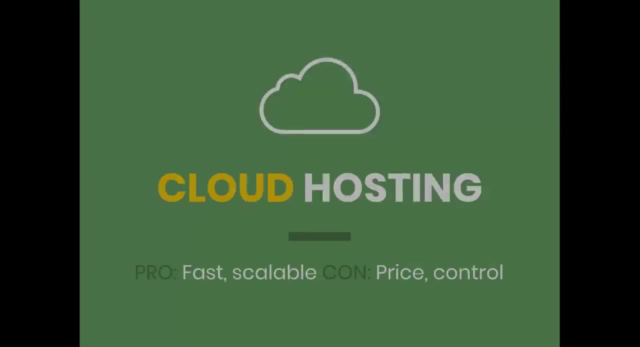 website and you're a technical host, So this is something that you're really only going to need if you have a high traffic website and you're a technical kind of person. Nowadays, a popular option is cloud hosting, So instead of your host being on a physical, 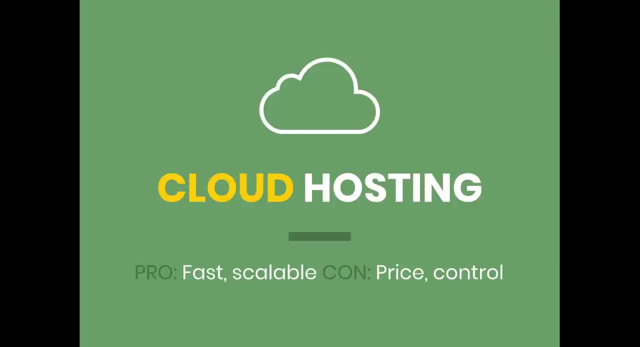 computer you know, sitting somewhere, maybe in the United States or internationally. your website hosting is on the cloud And the big advantage to this is that you have redundancy, So it's usually faster. It's more scalable, especially if the traffic surges start to. 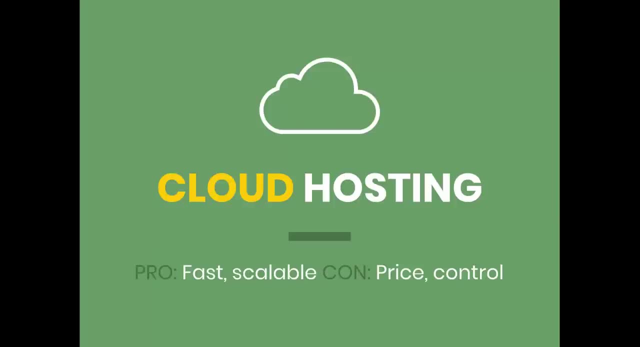 happen. You know your site's not going to crash as easily as it would if you were on a cloud, So this is going to cost you a little bit more, And the other downside is that you might not get the same access that you would if you had a dedicated server And a similar version of. 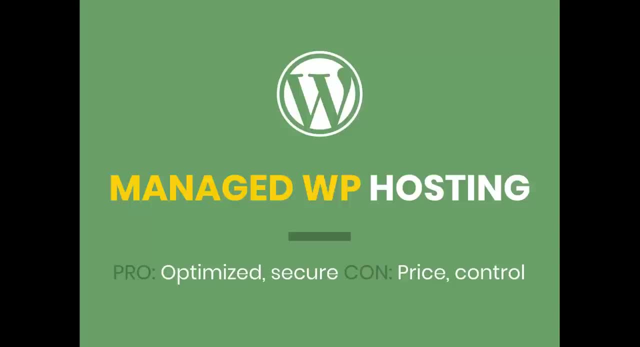 cloud hosting is managed WordPress hosting, So this is specifically optimized for the WordPress content management software and database-oriented websites. They also do a lot of updates for you, so it's going to be more secure. You don't have to worry about doing that manually. 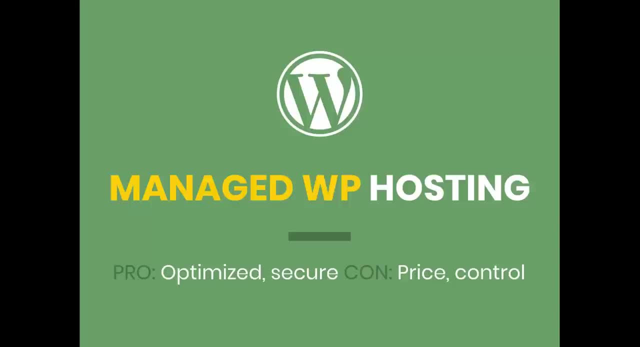 And similar to cloud hosting. the downsides to this are price and control, So I had to do this for one of my websites. It started to get a lot of traffic And the performance of all the websites that were on that shared server and that included both personal and client websites- the load speed. 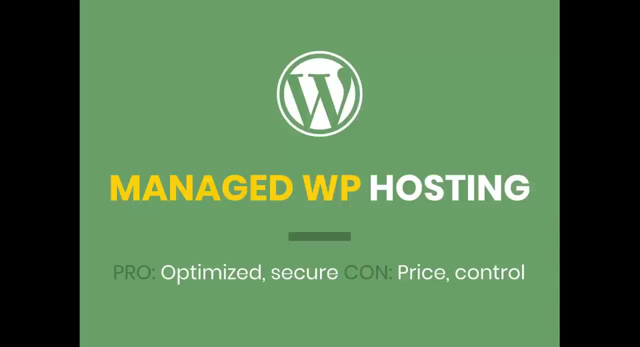 of all of them started to decline. So I knew I had to get my high-traffic websites off of that shared server and just keep the low-traffic websites on there. And when I switched over to managed WordPress hosting, I had to get my high-traffic websites off of that shared server. And when I 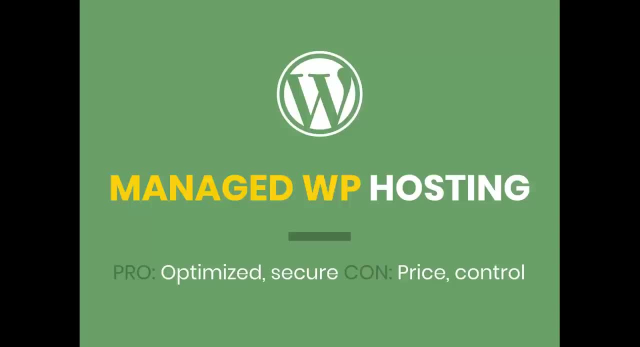 moved over to the Clara Go system and the company I chose was Kinstacom. the performance of the website just went through the roof. The page load time before was something between like a second to two seconds when I transferred over to Kinsta. it's now down to like point. 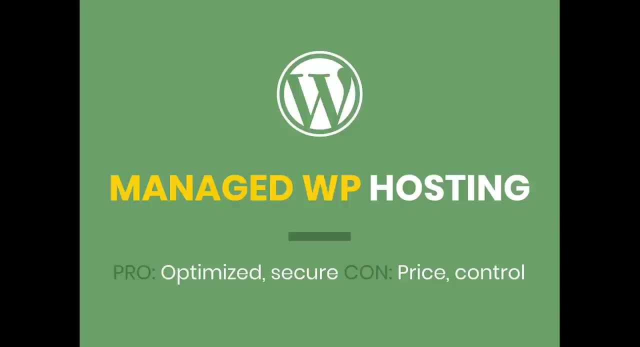 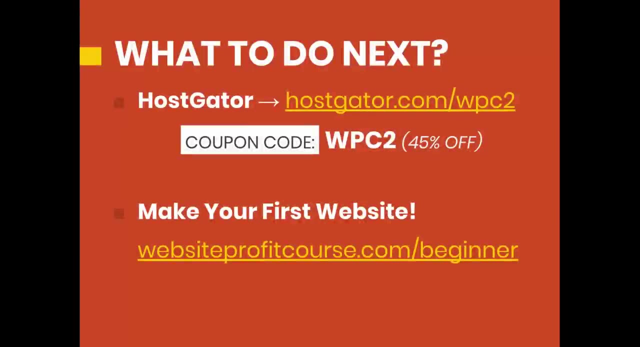 two seconds, So it improved way more than what I could have done by tweaking all the settings within WordPress or anything like that. If you're a beginner, though, don't worry about any of that stuff. Start with the most basic shared hosting package and get your website up, and 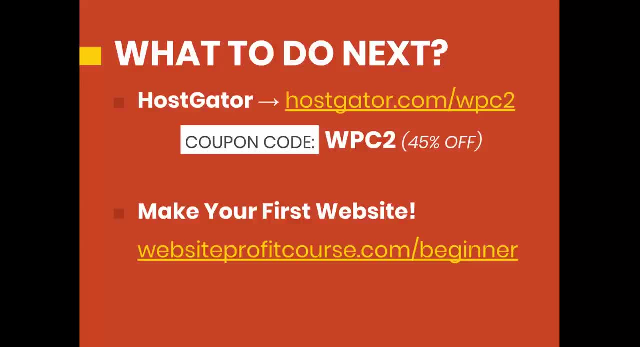 If you're ready to do that right now, I highly recommend HostGator. I've used them for almost a decade now, so they've been around a long time. They're very reliable and I think they've been one of the easiest to use. 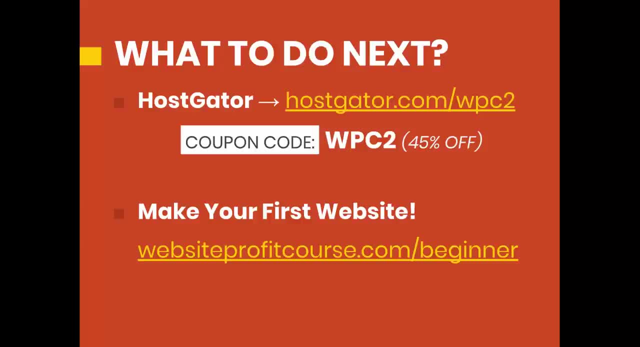 Go to HostGatorcom, slash WPC2.. I'm partnering with them to give you the best offer. for a one-year term, You'll get 45% off, and if you get to the checkout page in another way, you can apply this discount using the coupon code WPC2.. 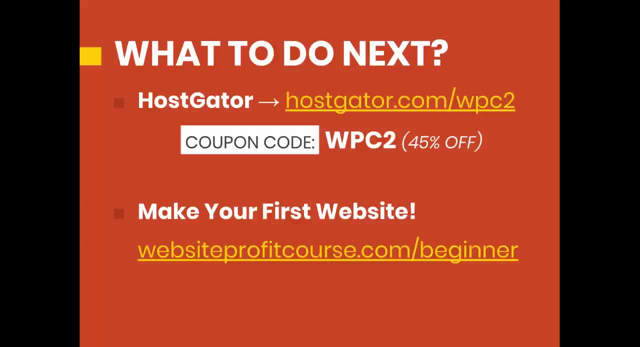 And if you don't have the time right now to set up your website, or maybe you just want a little bit more guidance, go to WebsiteProfitCoursecom slash beginner. I'm going to put together an email series where you'll get this video. 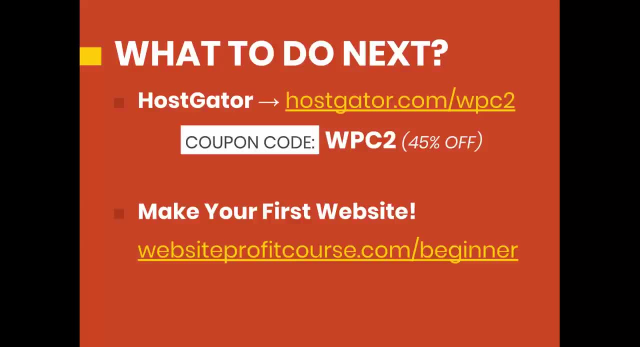 along with WordPress 101 tutorials so you can get accustomed to how to edit and create a website with WordPress, And on top of that you'll get a full-length tutorial, step-by-step, on how to create a business website from scratch.